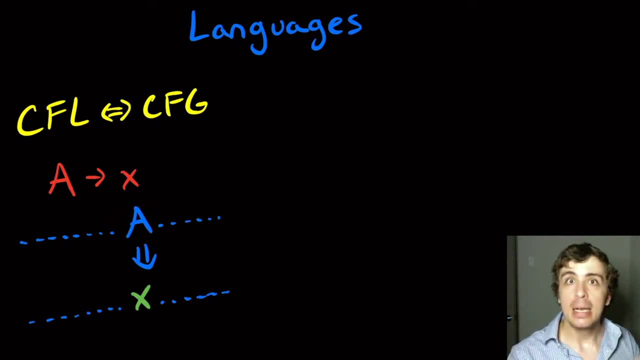 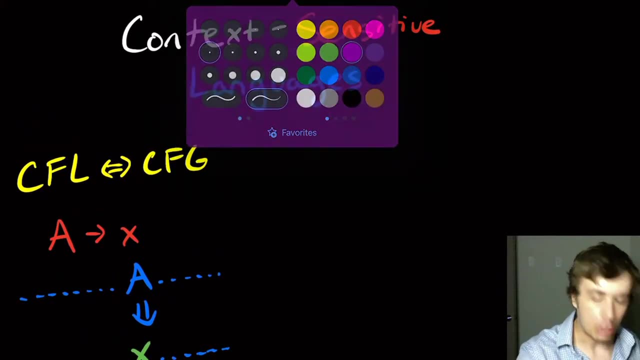 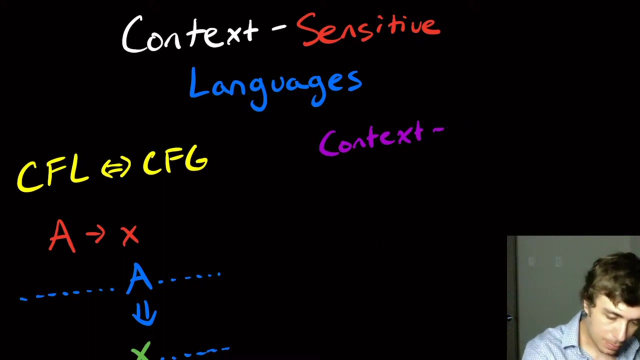 context of where this A actually is, in order to apply this rule in the first place. So that's what's called a context-sensitive language, and so there's an equivalent notion of a context-sensitive grammar. So let's talk about what a context-sensitive, let's learn to spell. 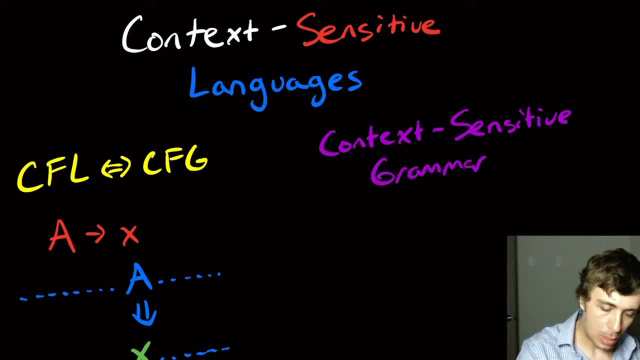 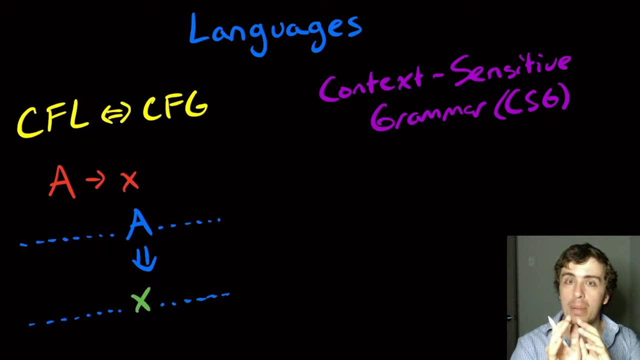 sensitive grammar or a CSG. So what is a context-sensitive grammar? Well, if you want to apply a variable replaced with something else, you need to know the context around it. So all of the rules are going to have a certain form, which is going to have some form. 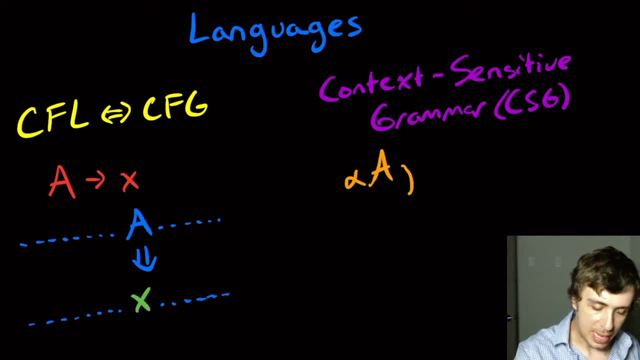 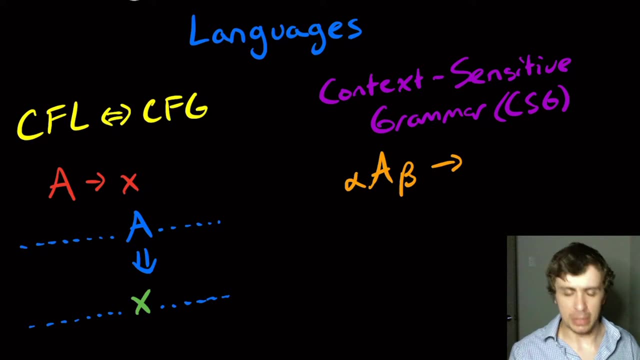 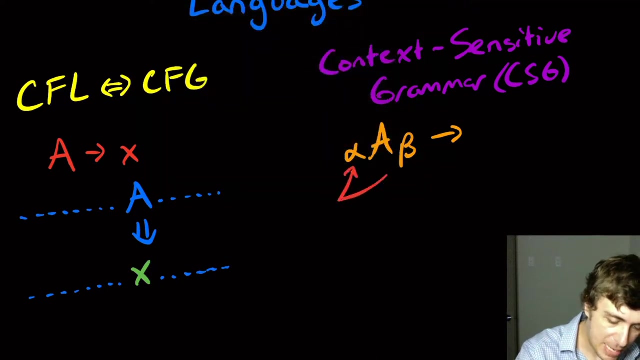 alpha, A gamma. Actually, I'm going to replace it, I'm going to say beta. here There are different notions depending on the textbook that you use here, But what we're going to have here is: this is the context. So the alpha and the beta here are the context in which the A appears, And we'll say: 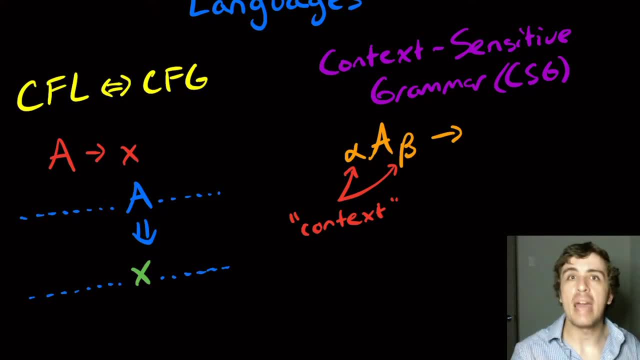 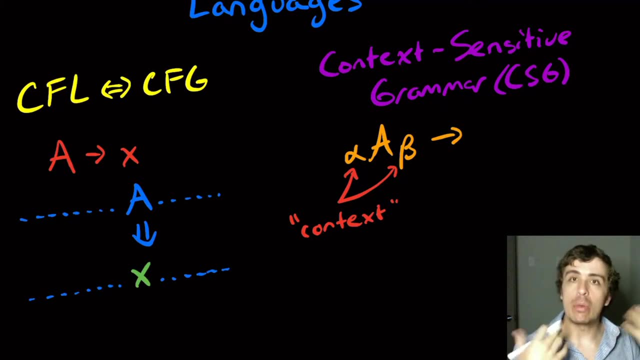 what alpha and beta can be in a sec. but that's what's around the A variable, And we don't want a context in which the variable occurs. It's just that we want to only be able to apply the rule in this particular context. So, whatever it's replaced with, let's just call it x, we have to. 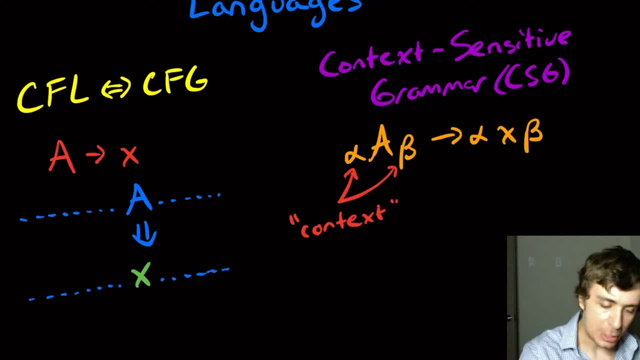 have alpha and beta on both sides of that too. So the context: wherever this A is, we're forcing it to under this particular condition. you can change the A to an x, but only under this particular condition. So we're going to have to have alpha and beta on both sides of that too. So the context. 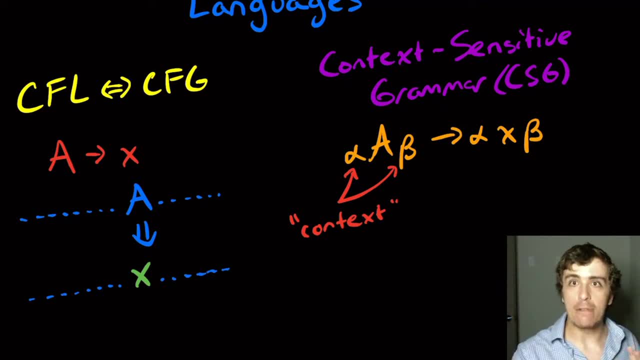 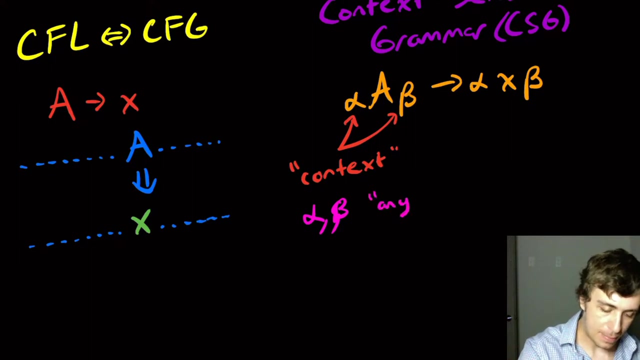 what it. so there are different notions of what these alpha and beta are, but the most common one is where we can have them be anything. The alpha and beta can be anything. So alpha and beta are anything, And we require that the x thing be non-empty. Okay, There's a whole technical 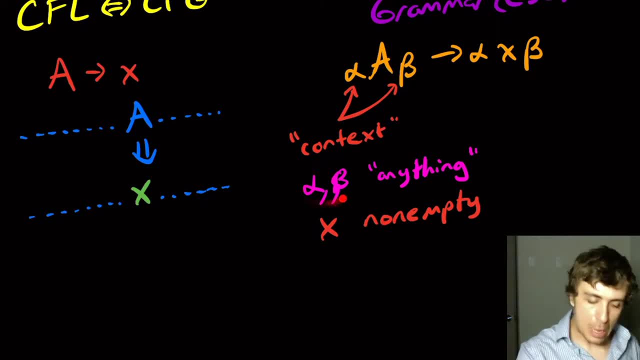 reason why that's the case. but you can have alpha and beta be anything that you want. In fact, they can be the empty string too. So, in fact, if we let alpha and beta be the empty string, then we recover the context-free grammar definition, because if there's nothing on both, 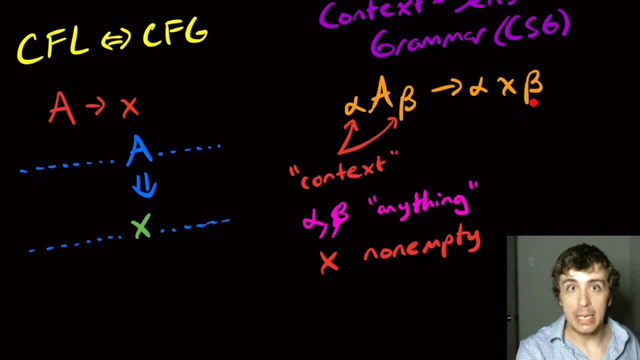 sides, it's the same thing as nothing on both sides over here too. So every context-free language is a context-sensitive language already, apart from this one-sided language. So if we let alpha and beta be non-empty, then we can have alpha and beta be non-empty, Okay. So that's one peculiar. 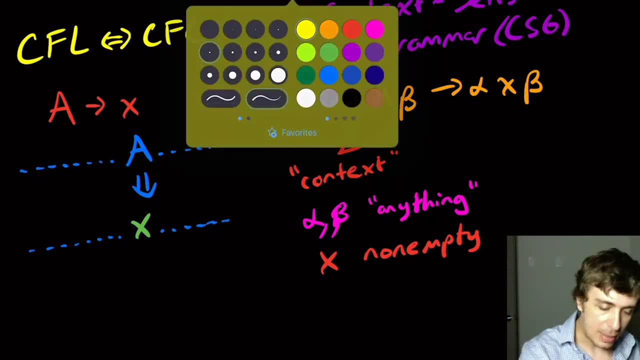 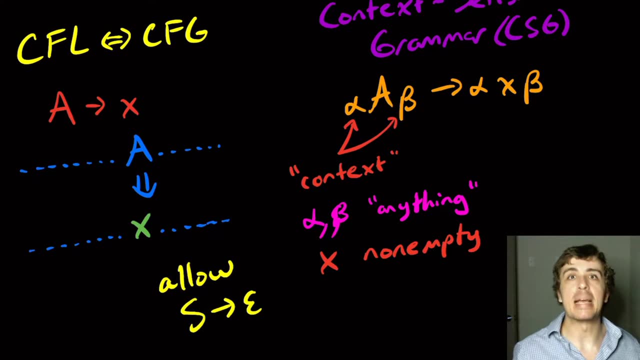 thing right here, where the right-hand side has to be non-empty because of this little condition right here. So sometimes we allow ourselves to have the start variable go to the empty string, as that's the only way to make the empty string and that will fix everything. So that implies: 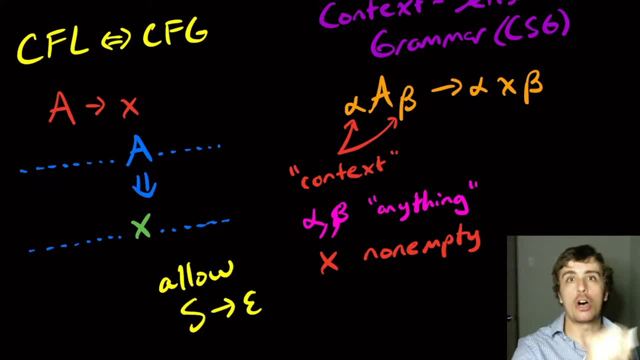 because these can be anything that you want. that implies that every context-free grammar is context-sensitive grammar, if we allow this, which is pretty cool. So let's think about: okay, well, if we have a context-free language, that's already a context-sensitive language. Let's. 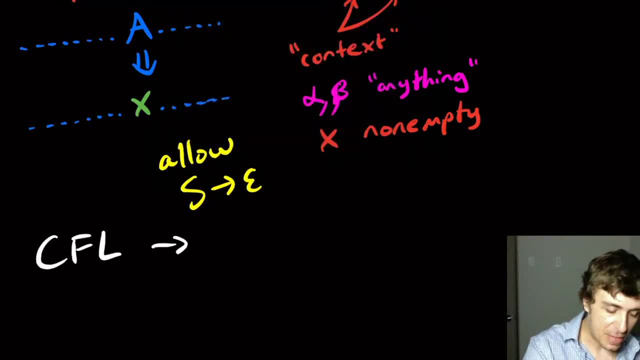 in fact write that down. So if it's a CFL, it already is a context-sensitive language. But what about the other way? So is every context-sensitive language also a context-free language? And I'm going to show you that that is not the case. 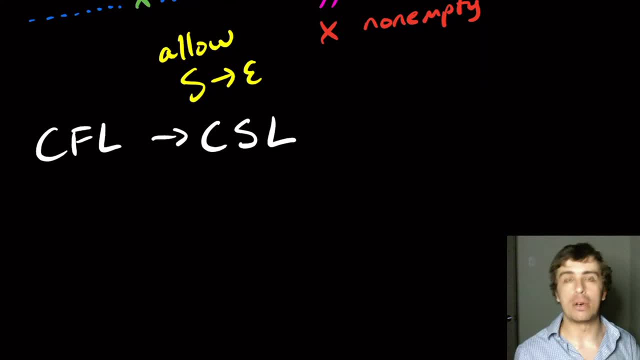 So we can have a context-sensitive language and we can have a context-sensitive language and we can actually make a context-sensitive grammar for something that is not context-free. And the prototypical language for this is A to the N, B to the N, C to the N, where N is at least. 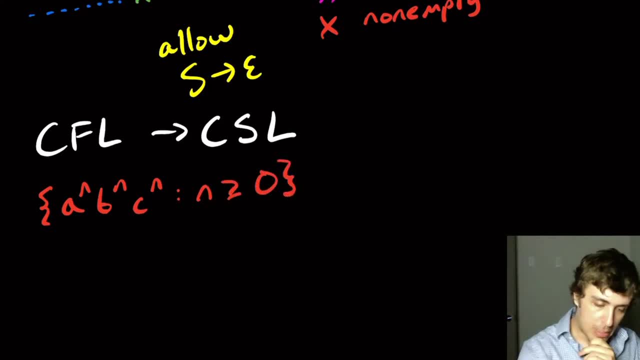 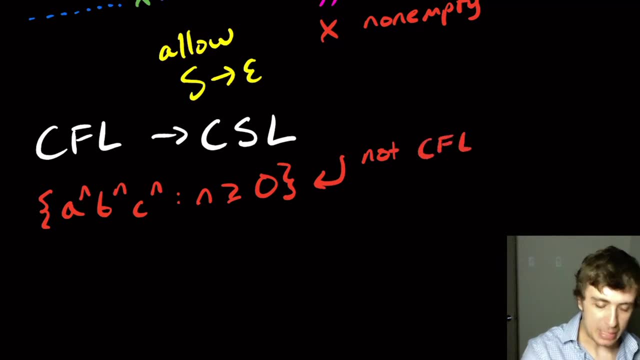 zero here. Okay, so here, this thing is not context-free, and I've done many videos on showing that this is not context-free, And what I want to show that is that you can make a context- sensitive grammar for this thing. So let's see. So how would we actually do this? Well, 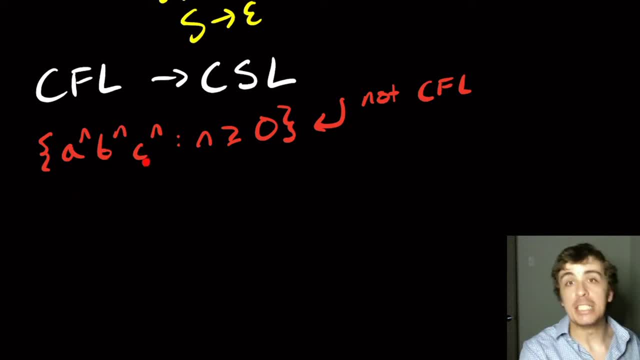 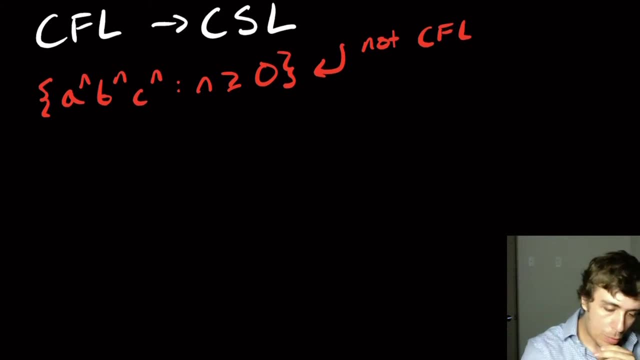 note that we have to have exactly the same number of A's, B's and C's all the way through. So what do we want to do here? So what I want to do is this. So let's have a start: variable make. 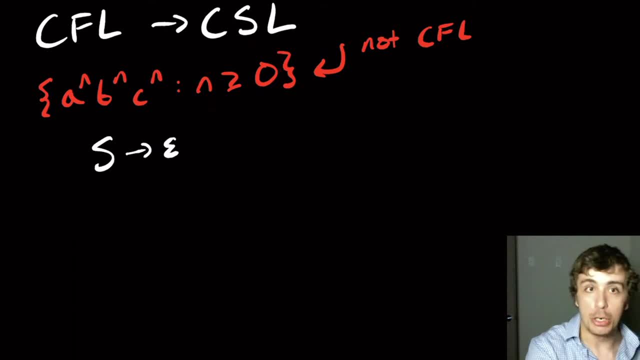 the empty string. So, in order to handle the zero case, and because that's the only way we can actually get the empty string according to this definition, So then, otherwise, what I'm going to do is I'm going to go to a variable S prime. So this guy is. 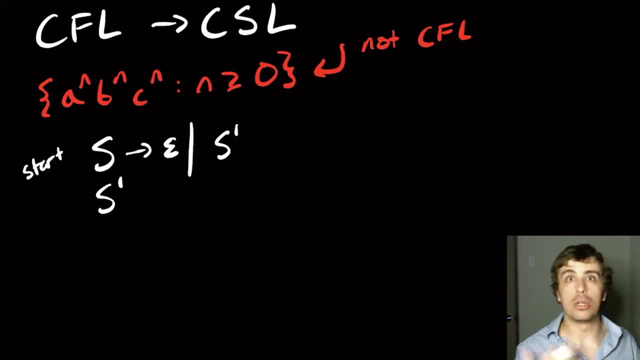 the start variable. So S prime is going to handle the non-empty strings in this language. Well, what are we going to do? Well, because the string is non-empty when we get to here, when we want to make it, and there are many ways that you can actually approach this, but if it's non-empty, 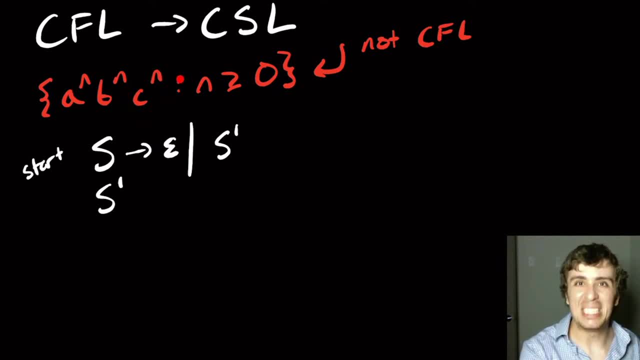 then obviously there's at least one C in the string. If we have a non-empty string in this language, we must have one C at least. So whatever this thing is, whatever it generates, it has to have a C at the end, no matter what happens before that. 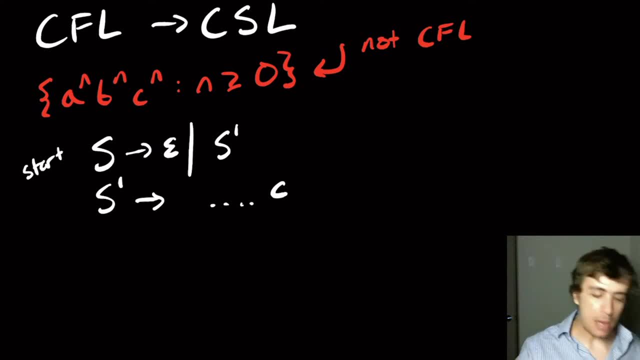 Well, let's see, what can we do. Well, we could have exactly one of the three characters, So exactly one A, exactly one B, exactly one C. So let's think about how that would work. So clearly I can just put A, B, C, like that. 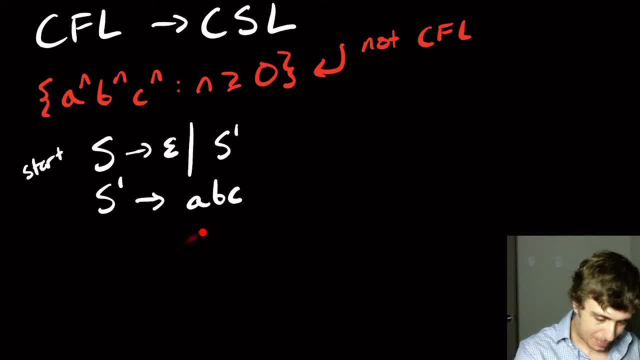 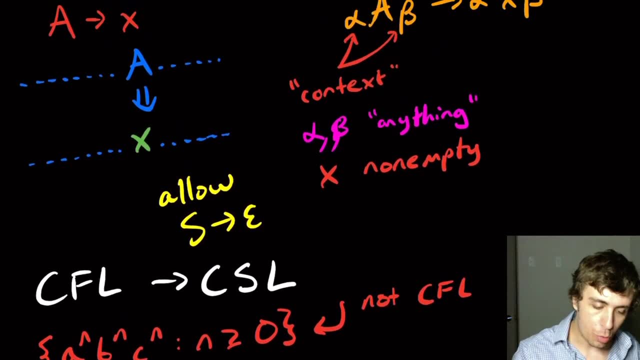 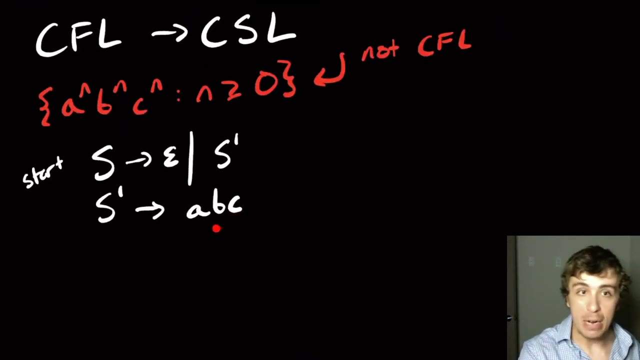 and then I can put C, B, C, like that. So that's going to help us a whole lot, because I can't insert any. sorry, according to the rules of a context-sensitive grammar, we have to have a variable in order to replace it with stuff, And this thing doesn't have a variable to replace it with. 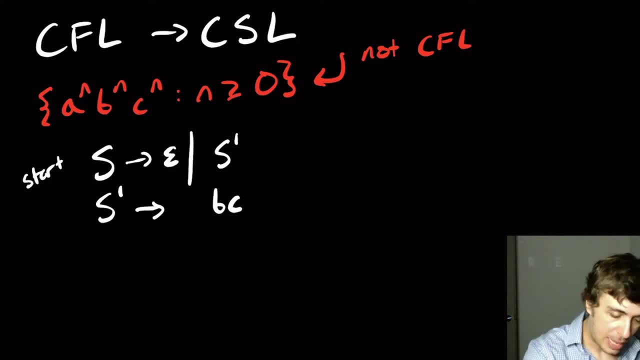 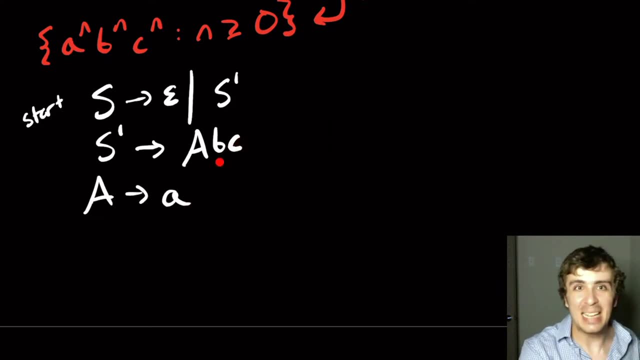 So what we're going to do here is we're going to have an A right there and then the A variable is going to make just a single A. So, in effect, I've done exactly the same thing, but I've done exactly the same thing, But this allows us to do more, because this inserts for us some context. 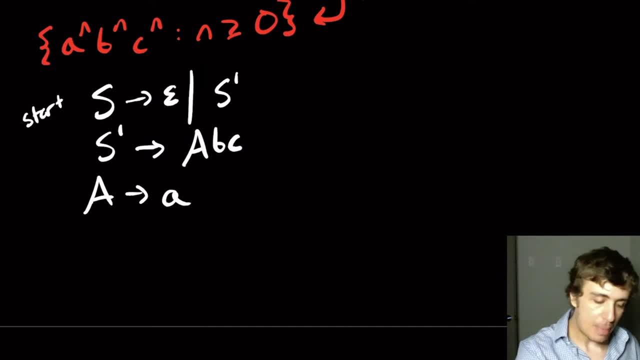 in order to have the A- B replaced with other stuff, Because, well, there's nothing over here which is allowed, but we have a B and potentially the C over here to replace it with. Okay, so what are we going to do here? Well, what I want to do is: let's think about 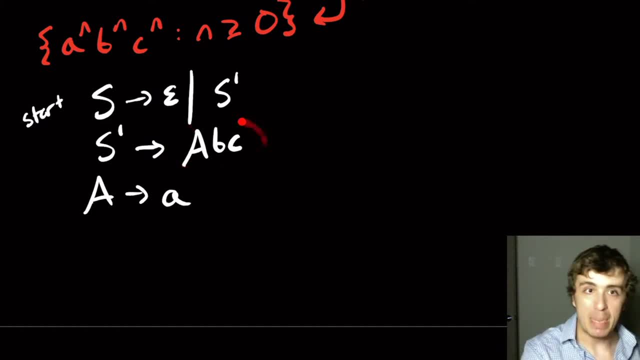 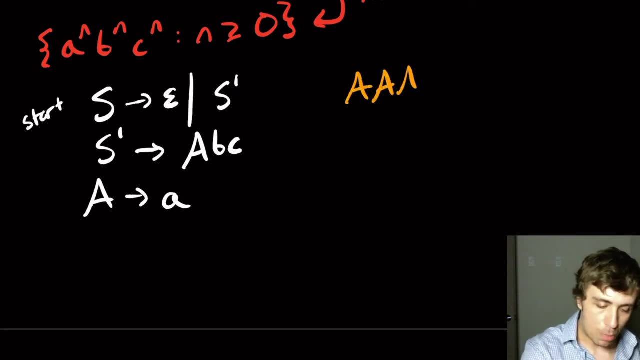 um, can we do something like this, which is a little bit more complicated? So what I kind of want to have is something along the lines of a whole bunch of A's variables, a whole bunch of B's, a whole bunch of C's as variables. 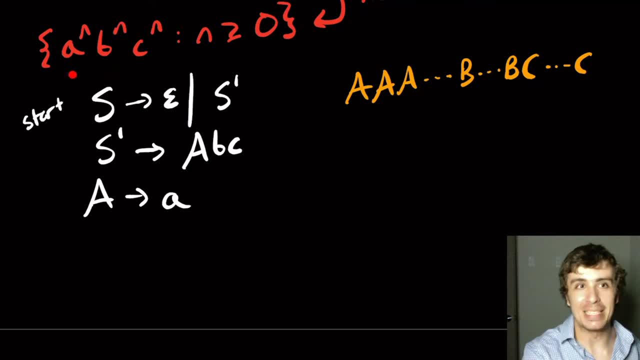 But this is equivalent to the original problem, obviously, because then I can just convert the A's, the capital A's to little a's, capital B's to little b's, capital C's to little c's, and we're back where we started. But what I'm going to do is not this, but I'm going to do. 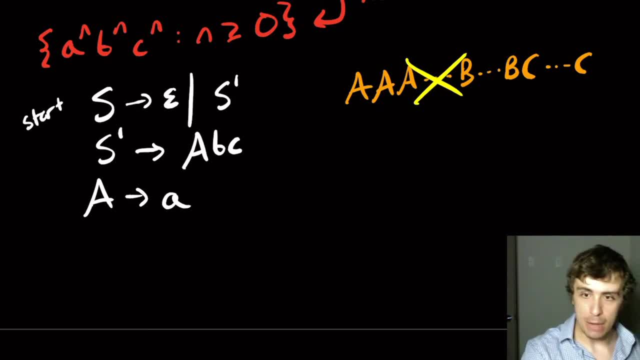 something very different. So I'm going to do something very different. So I'm going to do something very similar, which is to have A, B, A, B, A, B, et cetera, And then we have a whole. 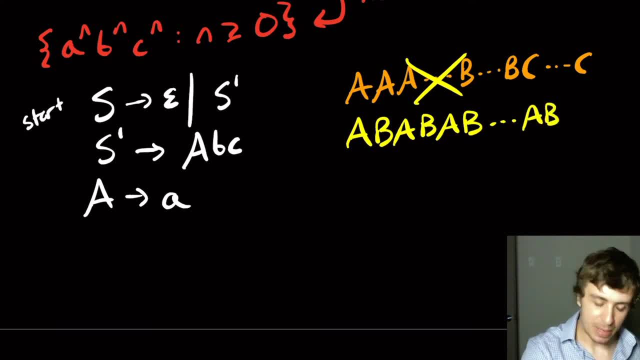 bunch of, let's just say, this ends with capital A, little capital B, And then I'm going to have a whole bunch of little c's at the end. Okay, So then why is this going to be a good idea? Well, what we're going to do is we're going to allow ourselves to swap the B? A's around. 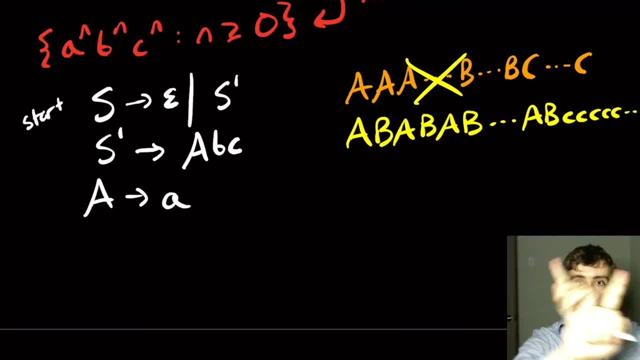 So the capital A's little a's, capital B's, capital C's capital B's, capital B's, capital B's, capital B, capital A, I'm going to allow ourselves to swap those, And so when we swap these, it's. 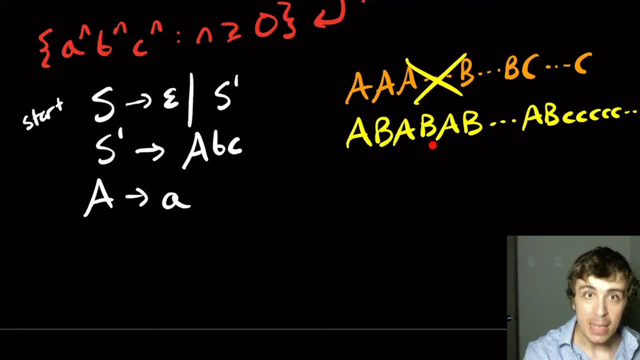 going to be capital A, capital A, capital B- B, And then we're going to have a B- A right here, And so we're going to allow ourselves to swap those and then swap the A further up if we wanted to, And then just keep going all the way through, And so that's exactly what this is going to do. 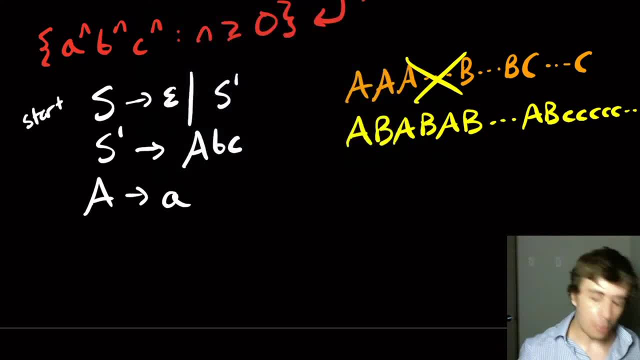 So one other rule for the S prime variable is to allow ourselves to have this A- B pattern. So what I'm going to allow ourselves to do is I'm going to have A, B, S prime C. So what this is in effect, going to do is it's going to make one C at the end for every occurrence of 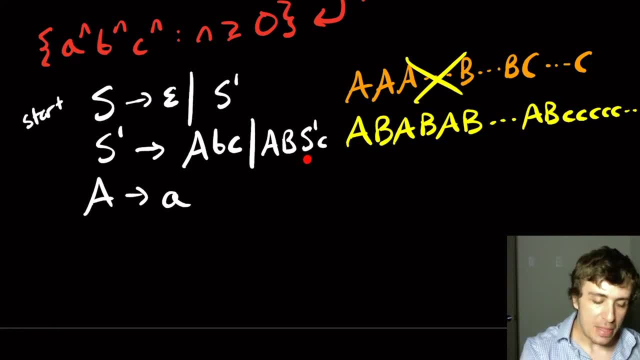 A and B- capital A, capital B- And then we're just going to recursively do that. So, effectively, the number of C's that I'm going to have here is equal to the number of capital A- capital B's. The only problem now is that the capital A- capital B's are in the wrong order. 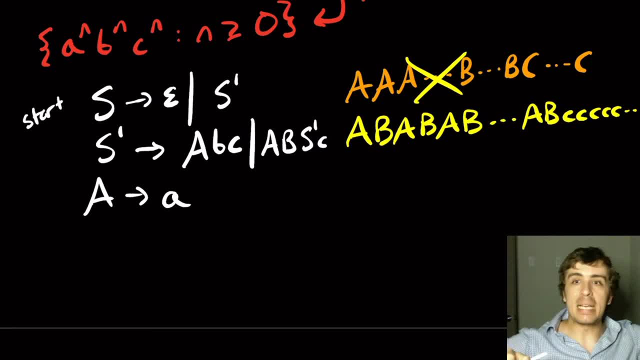 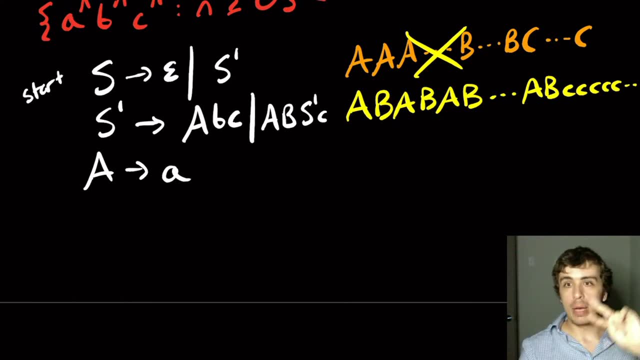 where I need to have the capital A's at the front and the capital B's at the end. So how are we going to fix that? Well, we can't just do a straight swap. We're going to have to do a number of swaps in the middle. So what I'm going to do in pink is the swapping part. 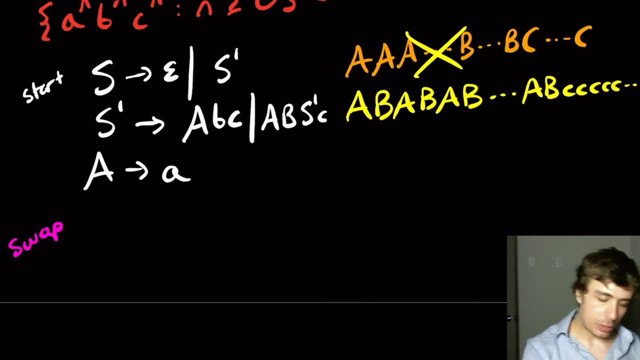 So here we're going to say, okay, we got to eventually turn the B A into a A B. That's what we eventually want. But what I'm going to do is I'm going to swap them a little bit at a time. 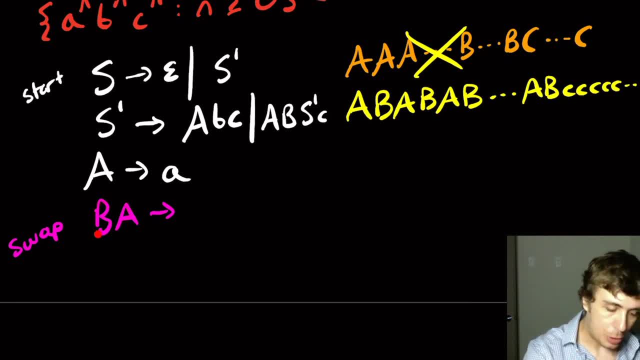 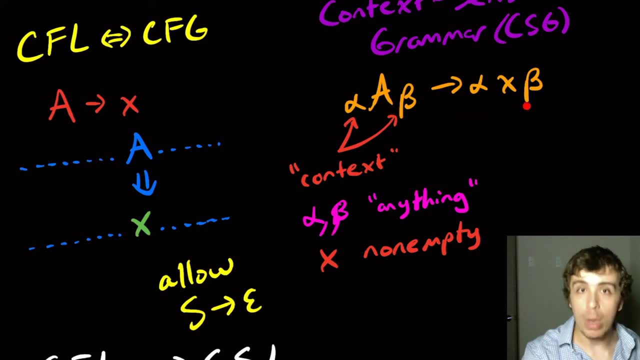 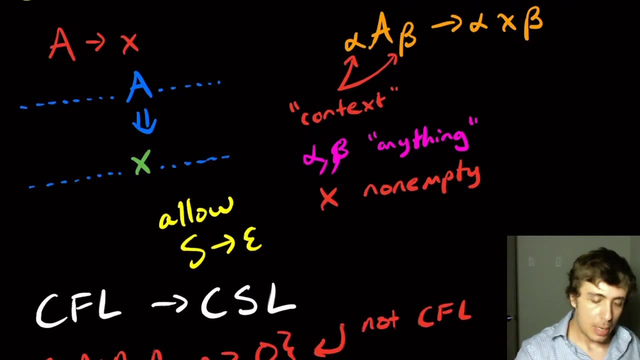 Okay, Because we can't just swap two variables at once. according to the definition, We can only replace one variable with another. So we're going to swap them a little bit at a time. The alpha and beta here can be terminals or variables if you wanted to, And in fact 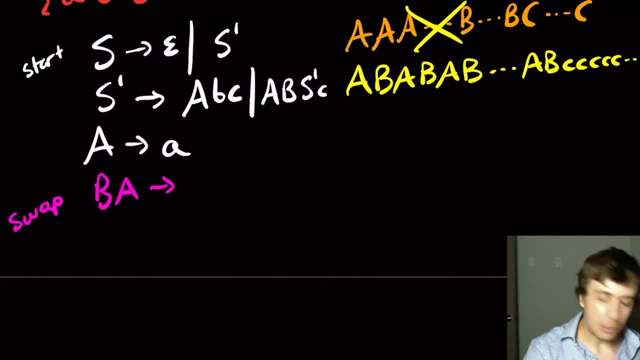 we're going to use that here. So here I'm going to allow ourselves to replace B A with capital C A, C A. I'm going to allow ourselves to replace with C B And then, finally, C B is going to be. 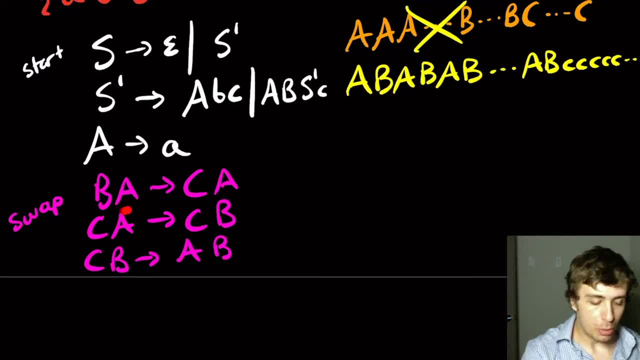 replaced with A B. So if I wanted to, if I allowed ourselves in the definition, I can just say: B? A gets replaced with A B And then finally, C? B is going to be replaced with A B. 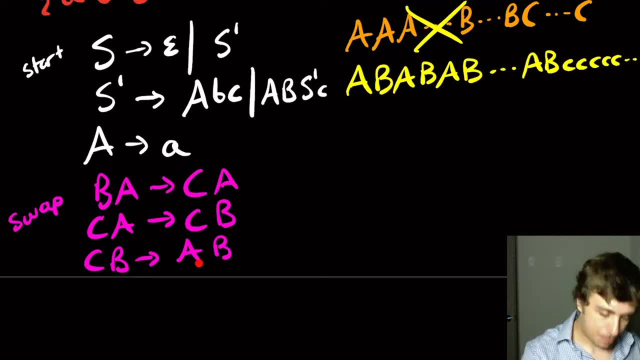 The problem with that is that we can't replace two variables at once, So we need to replace one at a time. So here I'm going to highlight the context. So the context is nothing on the left side of B and then the A. So then that's the context. It's the same context on both sides. 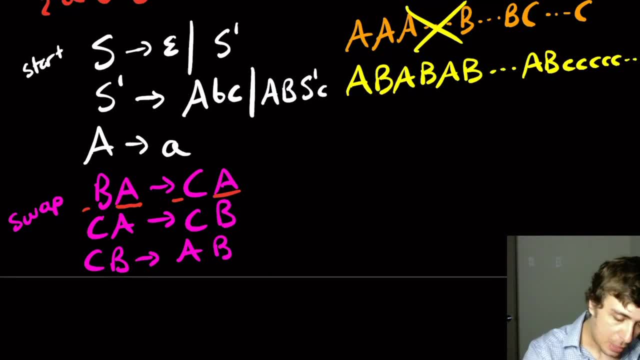 It's just replacing this B with a C, Then the context here is replacing the A with the capital B, And then the context here is replacing the A with the capital B, And then the context here is replacing the A with the capital B. So the context in the second rule is the capital C with 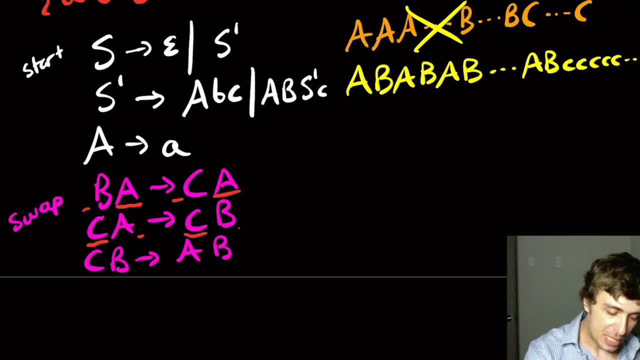 nothing on the right side, And then still C- nothing on the right side, And then the context for the final one is the B, with nothing on the left side. nothing on the left side, And then the right side is the context. Okay, So now we need to replace the Bs with- sorry, the capital. 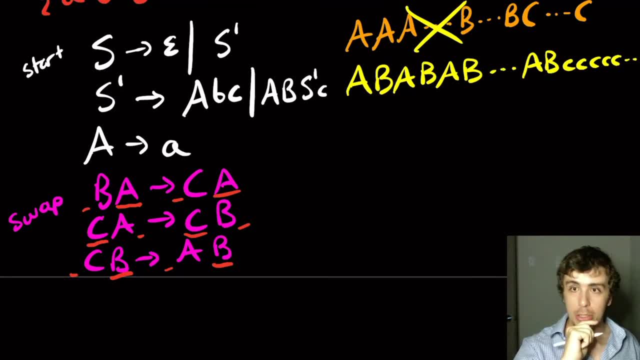 Bs with little bs. So then what we're going to do here is: well, if we're not in this rule right here, which will take care of that one B, we must have at least two Bs in the string. So then what I'm going to allow ourselves to do is to replace capital B little b.